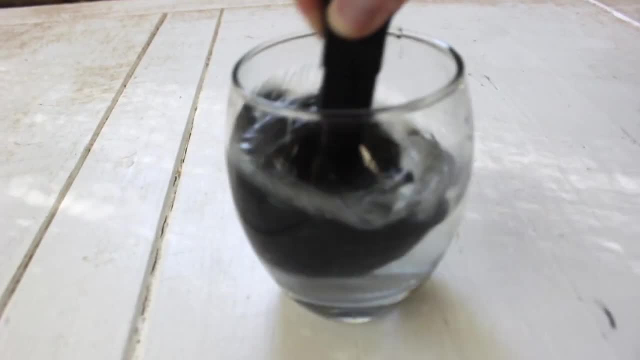 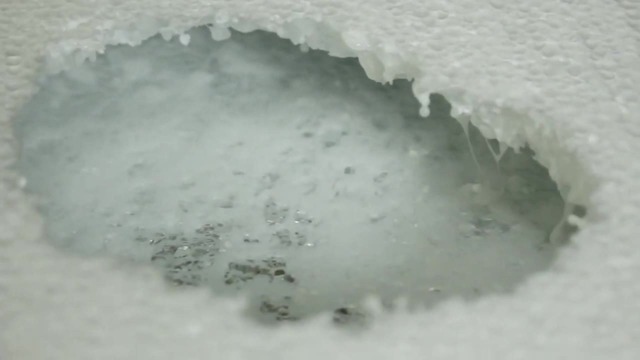 It's kind of like how water is good at dissolving sugar, making the sugar seem to disappear. Acetone is especially good at dissolving sugar. It's also good at dissolving styrofoam. It's so good, in fact, that you can make an entire block. 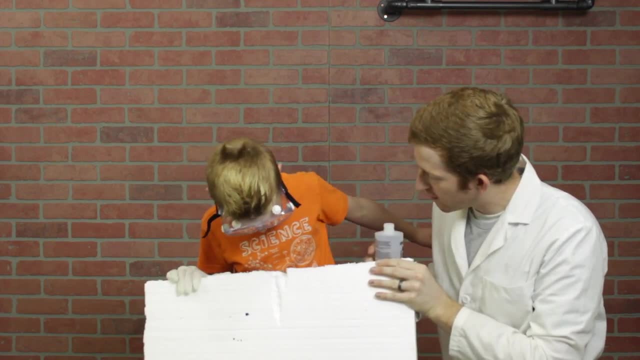 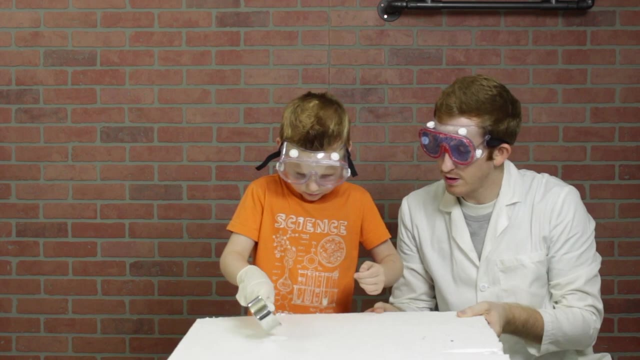 of it seem to disappear just by touching the two together. Wow, Yeah, you see that It's pretty cool, right? I can sit down here. Really, the acetone dissolves the styrofoam, making it seem to disappear. 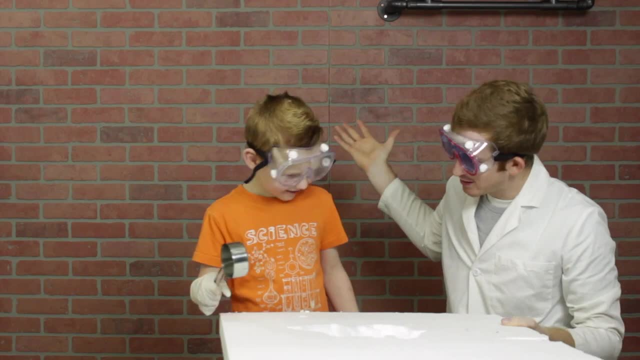 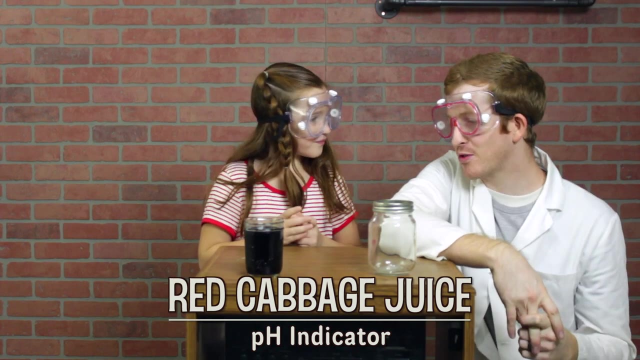 which releases all the trapped air in the styrofoam, And now it's all gone. Have you ever had cabbage? Don't know. Don't know, It's a vegetable and I don't think it tastes very good, But I'm sure it's healthy for you. 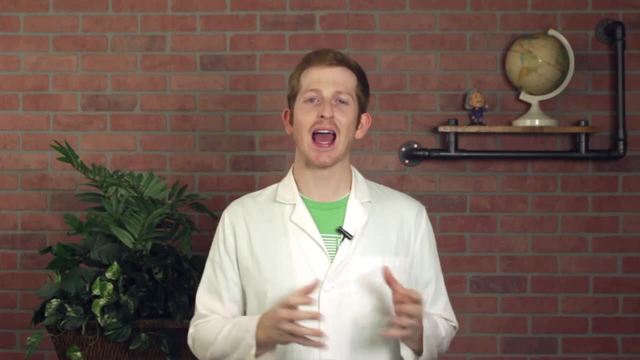 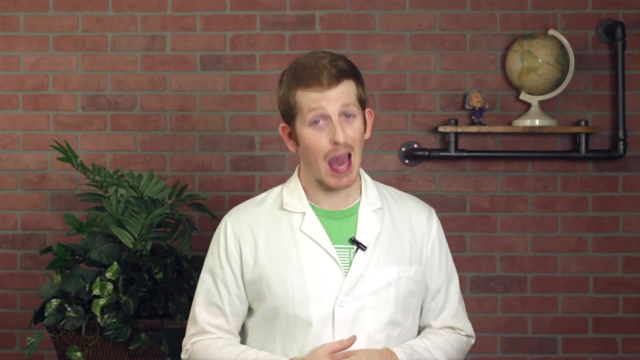 When we talk about the pH of something, we are saying how strong of an acid or base something is. But you can test the pH of liquids in your house with glorious red cabbage juice. Side note: this has to be the only good use of red cabbage. 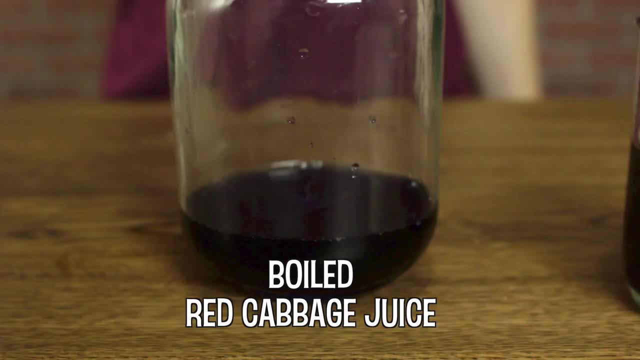 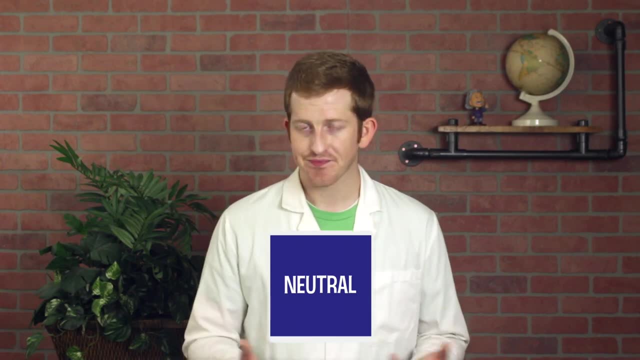 All you do is boil red cabbage until the water starts turning a dark bluish-purple. This color means the liquid is a neutral pH, meaning it isn't an acid or a base. It's in between. That's because all that is in the cup right now. 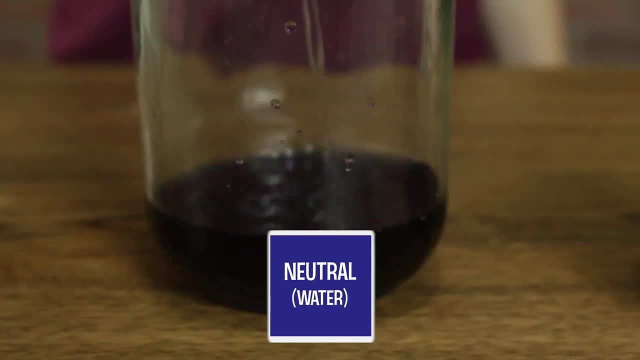 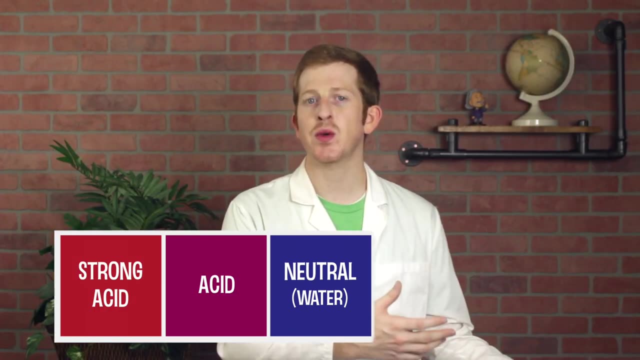 is red cabbage and water. Water is neutral. If the juice turns red when you add something, whatever you added was an acid. If it turns green or yellow, that thing you added was a base. Add any liquid you want to some of the juice. 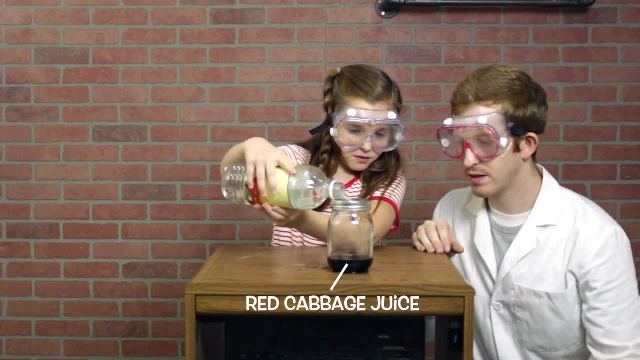 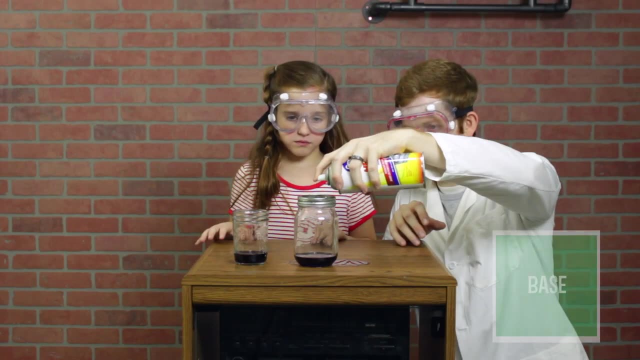 Liquids with little coloring work best. As we already mentioned, vinegar is an acid. If you add vinegar, the juice turns a red color. Cleaners are usually a base, so oven cleaner has a strong base in it, Yes, And it'll turn the juice green. 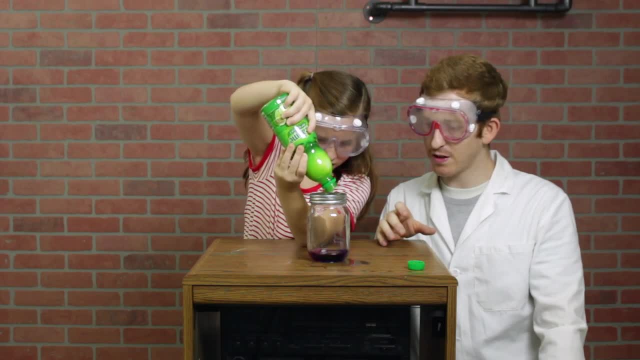 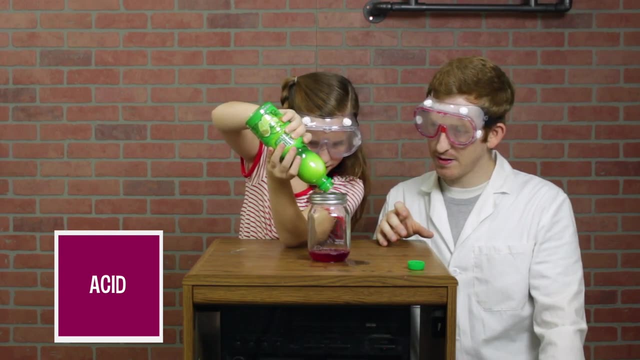 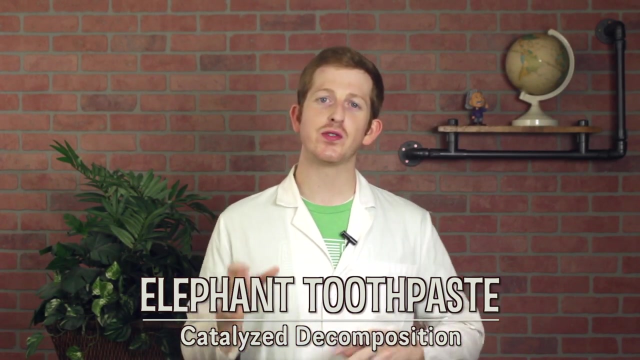 Acids are sour to the taste, so when we add some sour lime juice we see that it is an acid. Try it out and find out what things in your kitchen are acids or bases. Elephant toothpaste is a classic chemical reaction. A household version of it uses yeast. 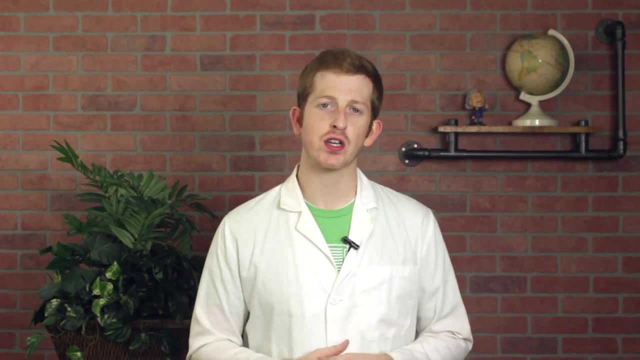 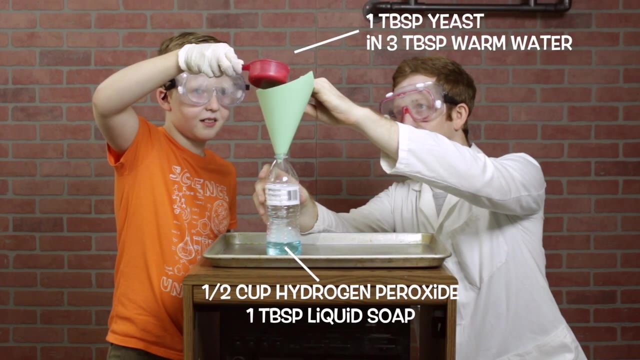 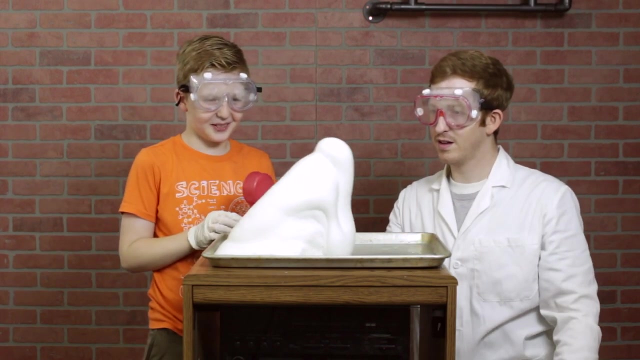 Remember, yeast is a living thing, It's a fungus. You can wake up these sleeping critters with three tablespoons of warm water and let them feast on half a cup of hydrogen peroxide. As the yeast eats the hydrogen peroxide molecules, it breaks them up, creating oxygen, gas and water.